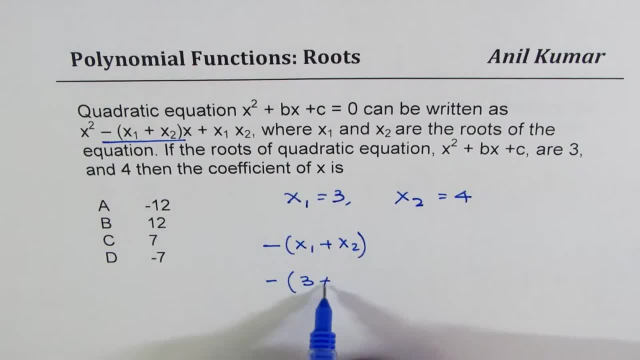 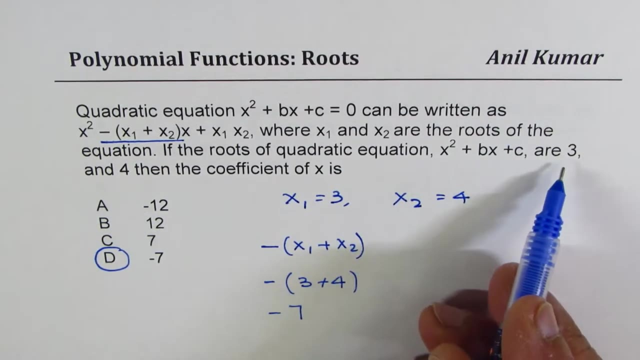 right. So it is minus 3 plus 4, which is minus 7.. So option D is the right option. okay, Now, if you don't know this formula, you could always get to the solution by writing. since you know that the roots are 3 and 4, you could say: 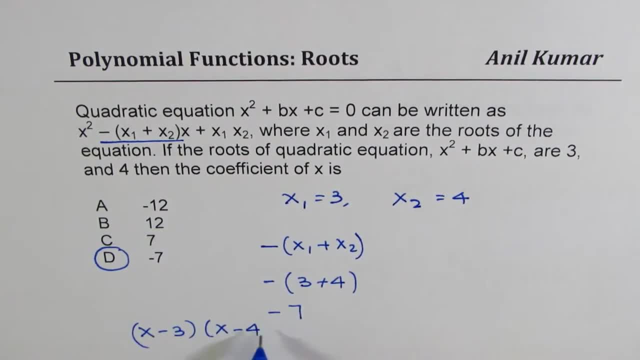 what is x minus 3 times x minus 4?? And when you expand, you get x square minus 4x minus 3x plus 12, which is equal to x square minus 7x plus 12.. So you again get the same answer, which is: 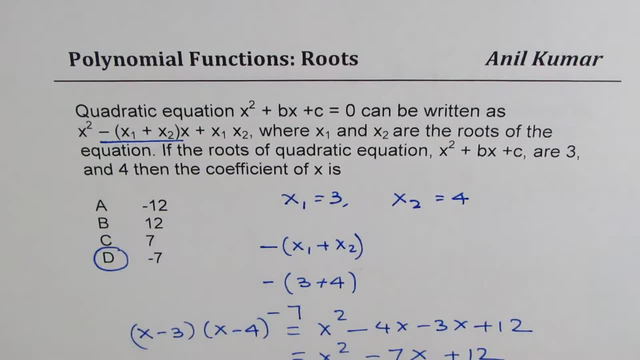 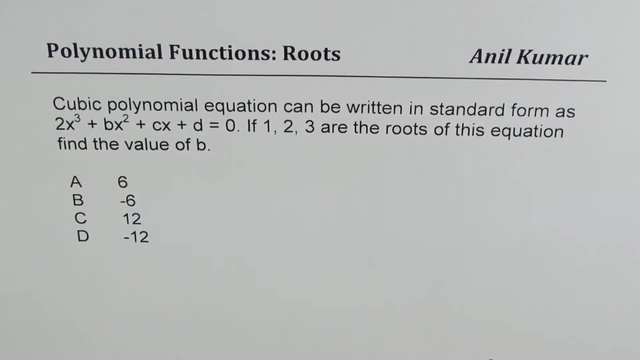 minus 7x, right. So if you don't know the formula, you can actually get to the result. That's important to understand. Knowing this, or having this information, gets you the answer in a few seconds. That saves a lot of time. Now here is the real question for you. Cubic polynomial equation can be written in: 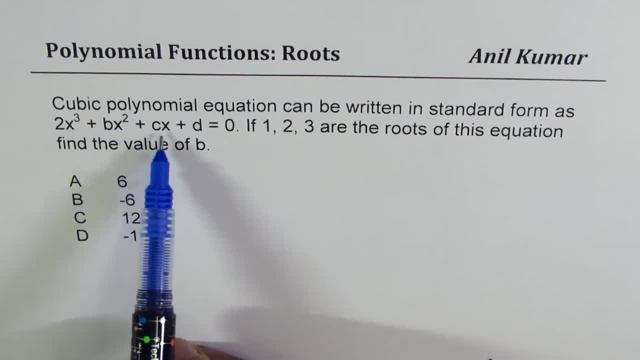 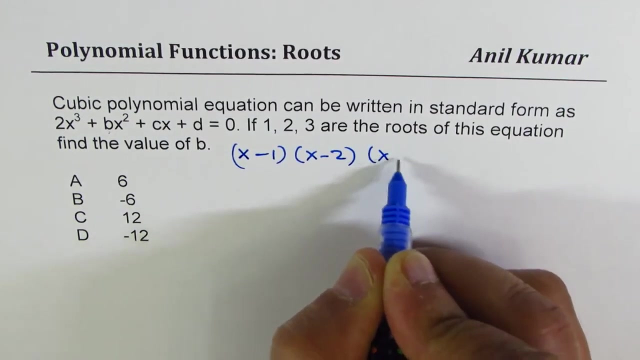 standard form as 2x cube plus bx square plus cx plus d, equals to 0.. If 1,, 2, and 3 are the roots of this equation, find the value of b which is coefficient of x square. Well, one way is that you could always expand x minus 1 times x minus 2 times x minus 3 and find 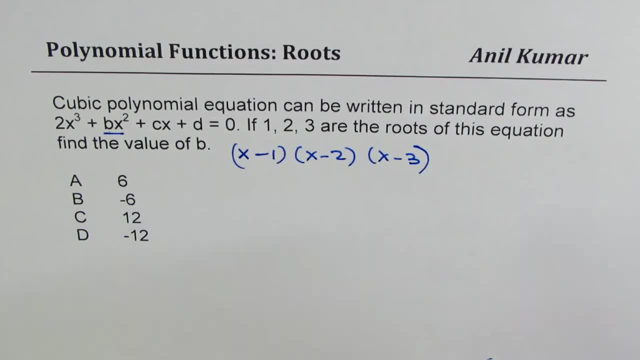 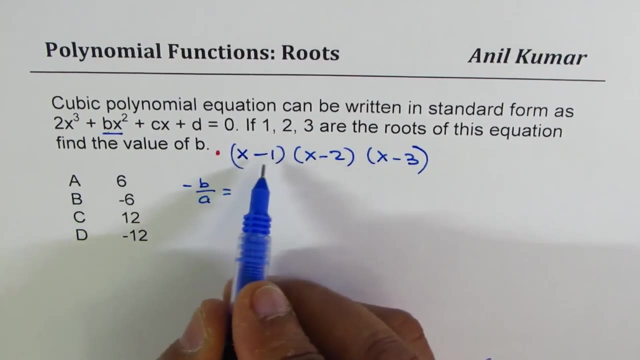 the coefficient of x square right. The other method is to use the formula. I like you to derive the formula so that it can help you to solve similar questions. The formula is that minus b by a is equal to sum of these roots. 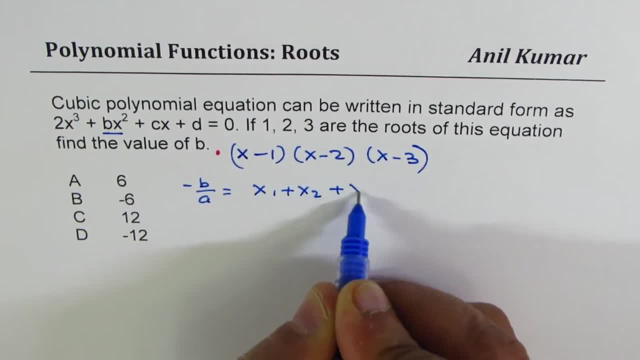 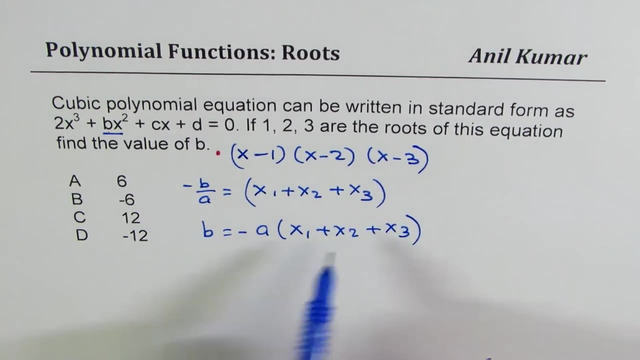 That means x1 plus x2 plus x3, right Sum of all three of them. So you can find coefficient of b as equals to negative a times x1 plus x2 plus x3.. In our case we know a is 2, so we'll write. 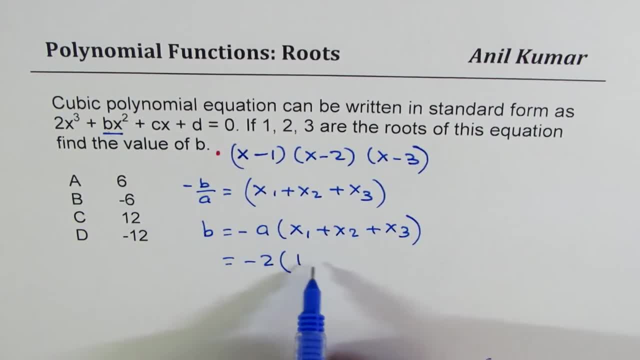 negative 2 times x1, x2, x3 are the numbers 1 plus 2 plus 3. And that gives you negative 2 times x1 plus x2 plus x3. And that gives you negative 2 times x1 plus x2 plus x3. And that gives you: